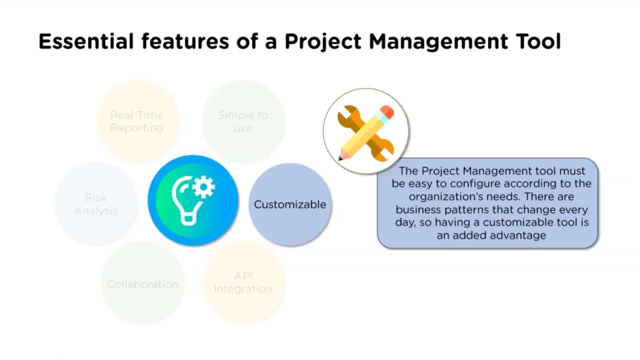 needs every project management approach. every project management templates. every artifacts needs technical support. Each project management tool needs enough in adoption before adopting as part of the practice. There are business patterns that change every day, so having customizable tool is an added advantage. 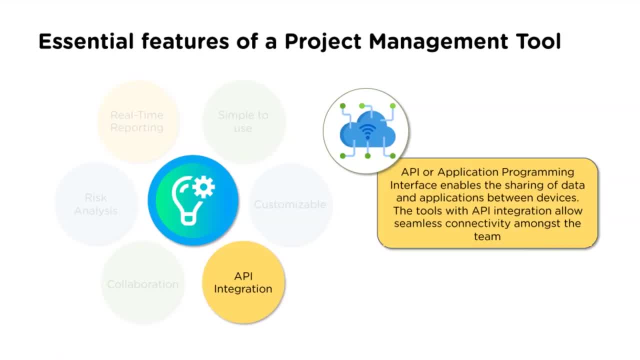 API or application programming interface enables the sharing of data and application between devices. The tools with API integration allow seamless connectivity amongst the team. The project management tools must allow for collaboration so that whole team can work together. Collaboration not only makes that task easier, but also increases the productivity of the 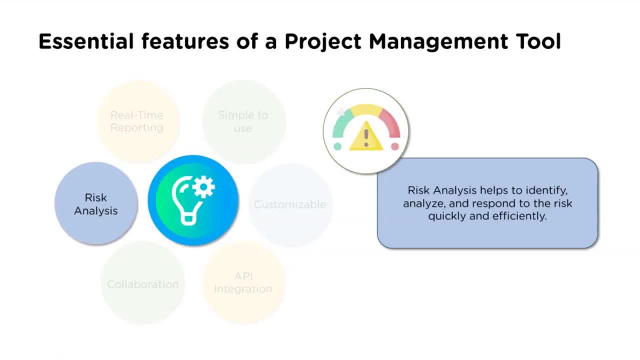 project Risk analysis helps to identify, analyze and respond to the risk quickly and efficiently. It needs to capture all the details of the risks, their impacts, the probability of occurrence of the risk and risk responses, and tracking them throughout the project lifecycle. The real-time reporting enables the 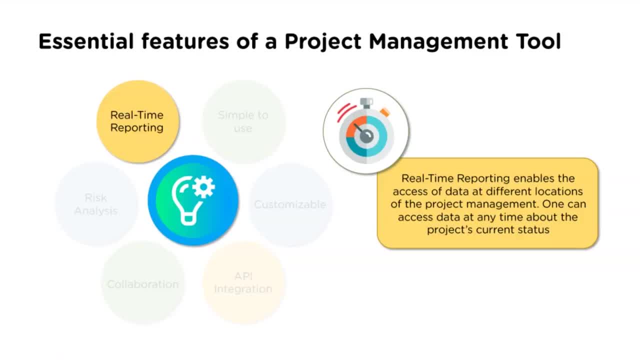 access of data at different locations of the project management. One can assess or access data at any time about the project. The real-time reporting allows the project manager to monitor the project's current status. This will help in having a real-time update about the 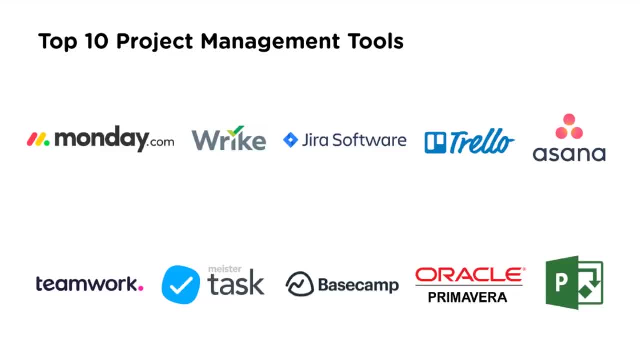 project status to the stakeholders of the project. The top 10 project management tools. what we have today in the market are Mondaycom, RIC, Jira Software, Trello, Asana, Teamwork, Meistertask, Basecamp, Oracle's Primavera and Microsoft. 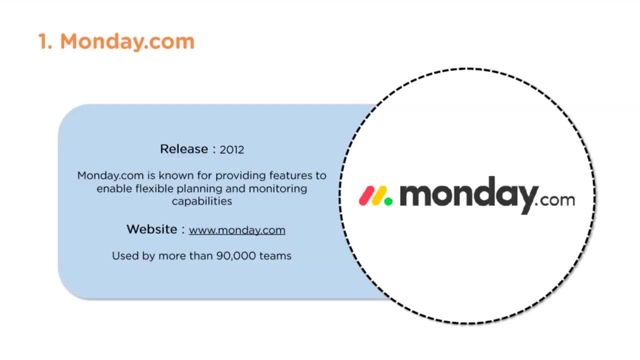 project management tool. So let us look at these one by one. So Mondaycom was created in 2012 and it is known for providing features to enable flexible planning and monitoring capabilities. The website where you can find Mondaycom access the tool is wwwmondaycom, So this tool is used by more than 90,000. 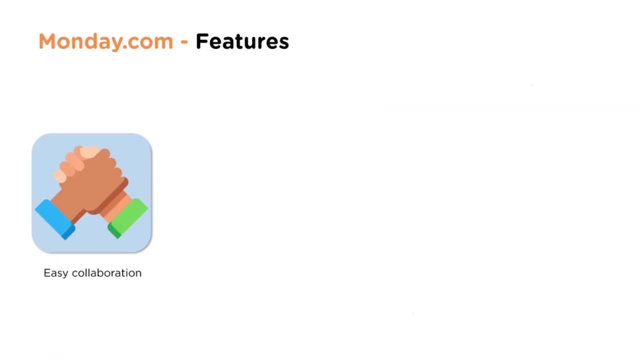 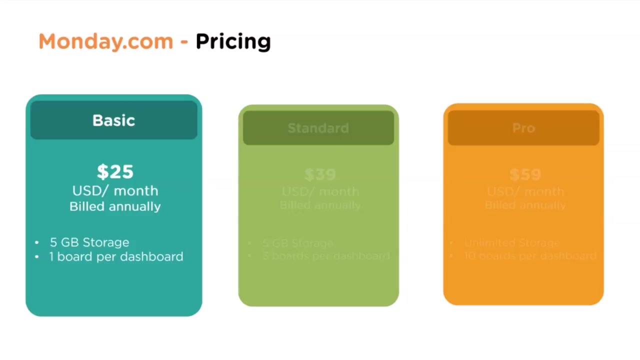 team across the globe. Mondaycom features and functionality includes: it is easy for collaboration, highly customizable, excellent for analytics, integration with Dropbox, Google Drive and Pipedrive. so pricing: the basic version is $1.25 on monthly basis, so which will provide you. 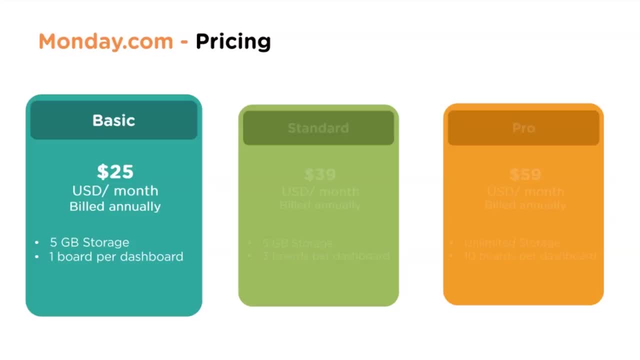 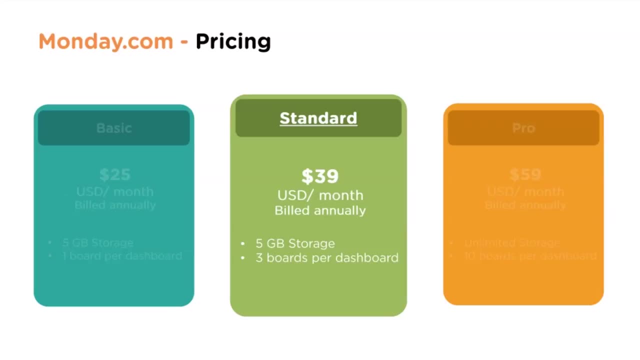 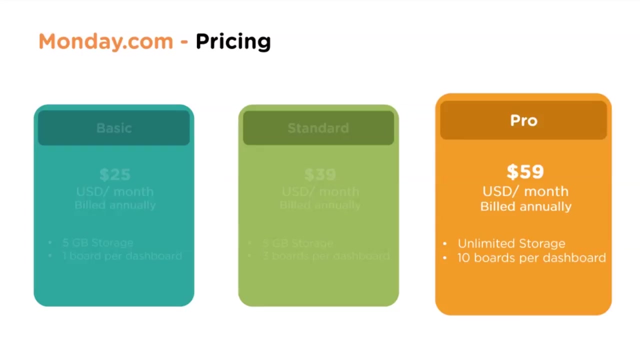 5 GB storage, one board per dashboard, and it is billed annually. The standard package includes 5 GB storage, three boards per dashboard, and it is $39 per month, which is billed annually. Professional includes unlimited storage- 10 boards per dashboard- and it costs $1.59 per month and it is billed annually. Mondaycom is used by the market to provide any different infrastructure like 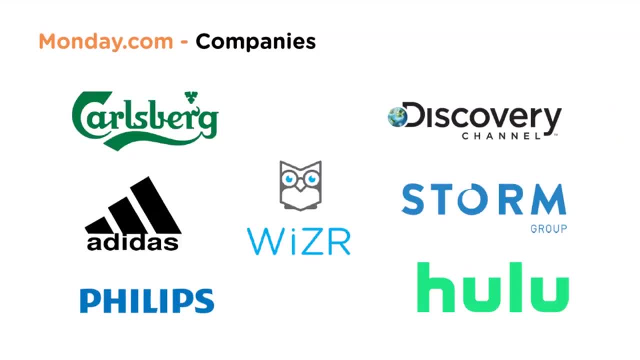 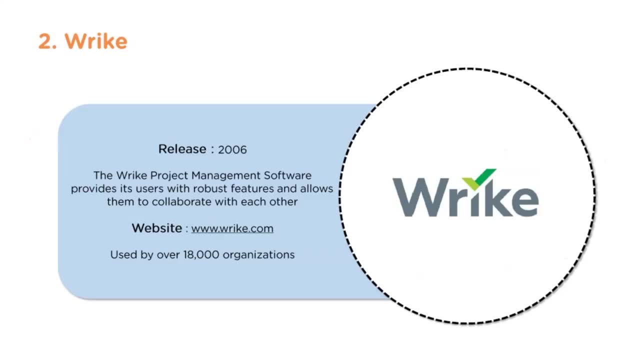 the following: customers: organizations of mondaycom, that is, girlsburg discovery channel, adidas, tom phillips, etc. rick is another project management tool which was released in 2006, so this application provides its user with robust features and allows them to collaborate with each other. the website to. 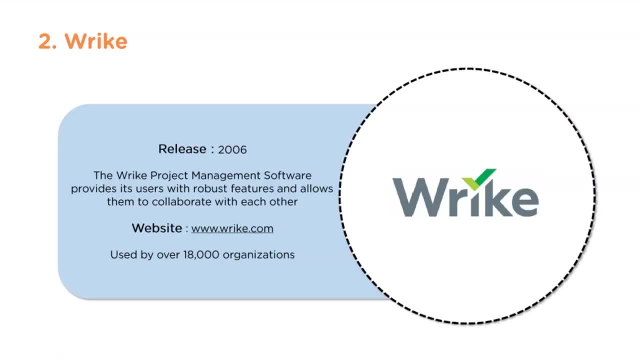 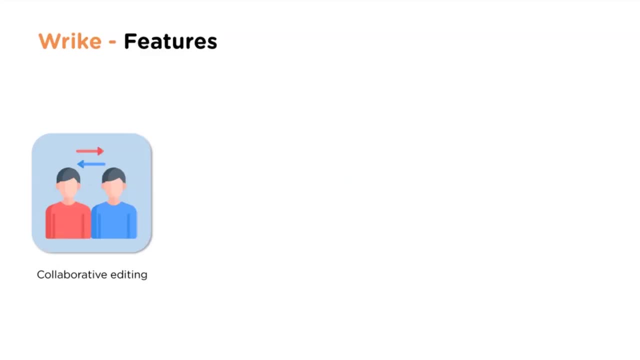 access. the tool is wwwreccom and this is used by over 18 000 organizations across the globe. the features of rig includes: it has collaborative editing, flexible workflow, real time reporting and efficient work management. the pricing includes 0 to 5 users. it has basic integrations and which. 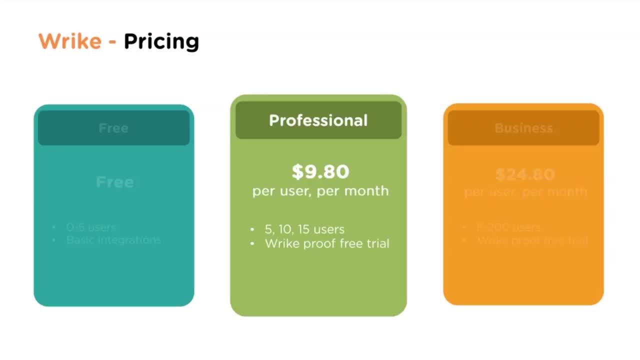 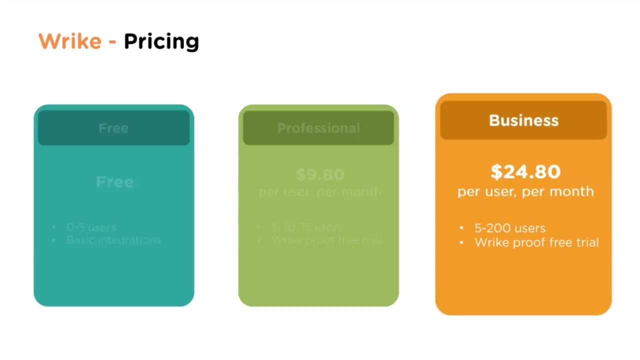 is free, whereas professional includes dollar 9.8 per user per month, which is, which has a slabs of 5, 10 and 15 users, and reek proof free trial. business version has 5 to 200 users and rick proofji free trial, whereas 24.80 dollars per user per month. the companies which uses the rig tools are: 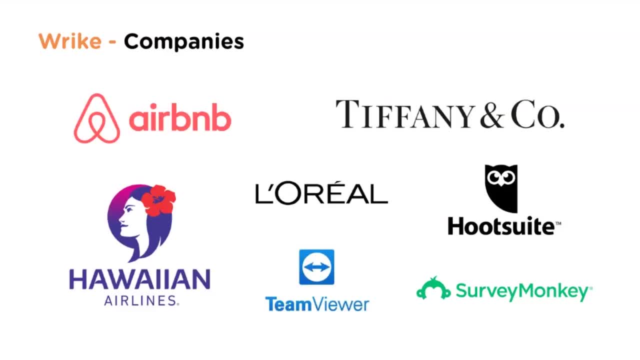 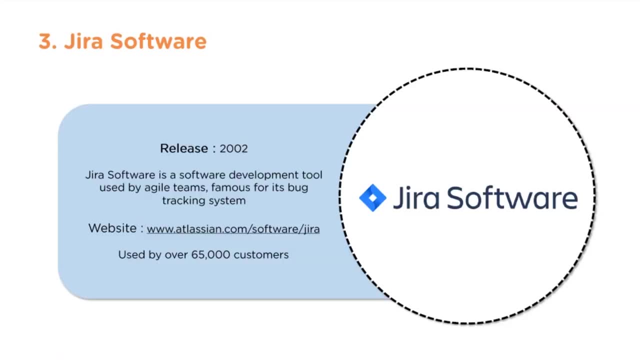 airbnb, laurel team, viewer tiffany and co, etc. now let us look at jira software. jira software was released during year 2002. it is a software development tool used by agile teams, famous for its bug tracking system. the website to access this tool is www dot atlaciancom software jira. 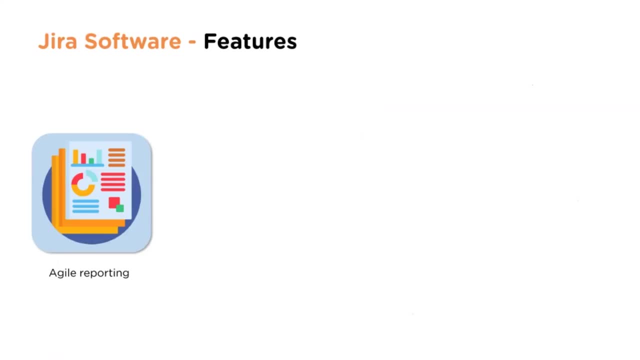 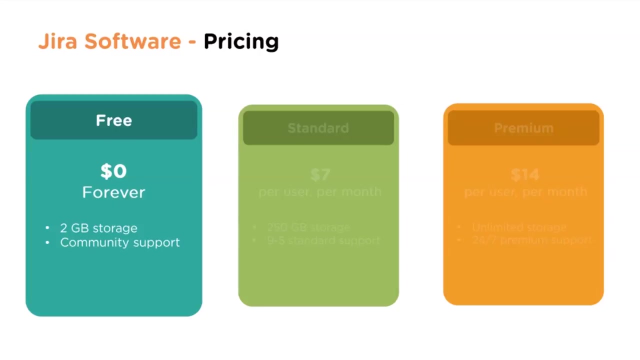 used by over 65 000 customers. the features of jira software includes agile reporting, rich tool kit for developers, bug tracking, mobile applications. so the pricing of jira software is as follows: so for forever, 2gb storage and community support which cost dollar zero. but 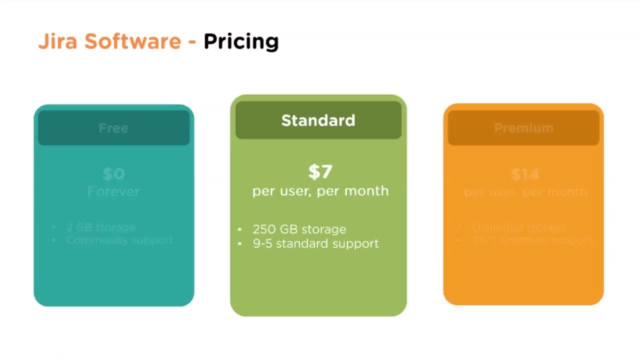 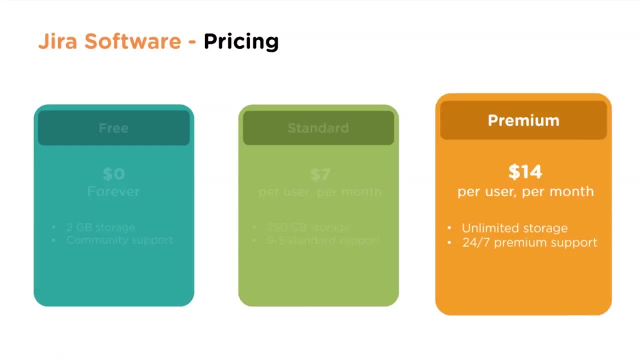 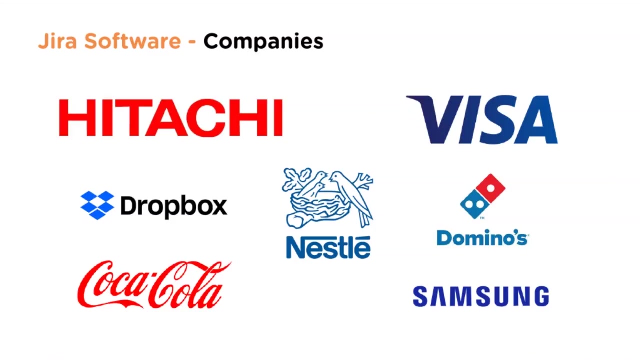 a standard azure $7 per user per month, which includes 250 GB storage and 9 to 5 standard support. premium is $14 per user per month unlimited storage and has 24 bar 7 premium support. Jira software is used by the organizations. that is Itachi Visa. 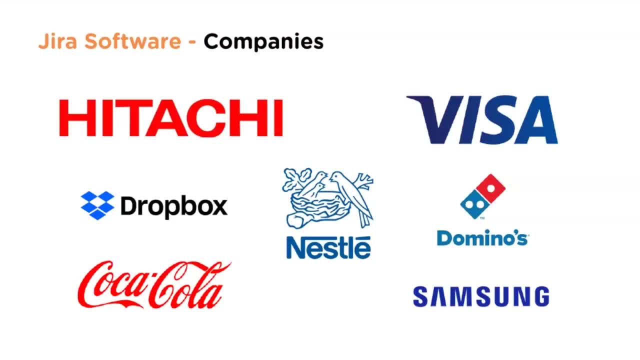 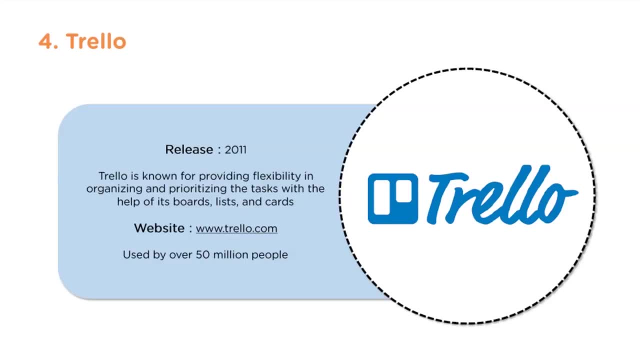 Dropbox, Nestle, Domino's, coca-cola, Samsung, etc. now let us look at the tool, Trello. so this application was released in 2011. it is known for providing flexibility in organizing and prioritizing the tasks with the help of its boards, lists and cards. website to access the tool is wwwtrellocom. 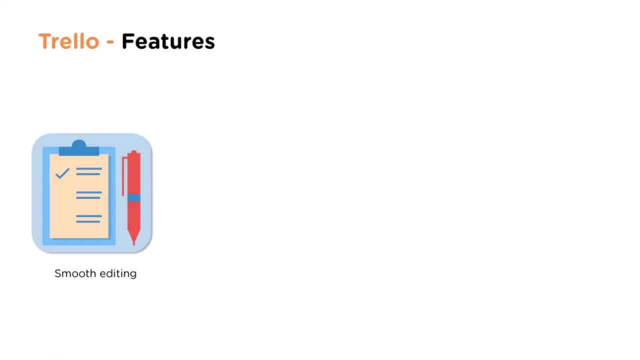 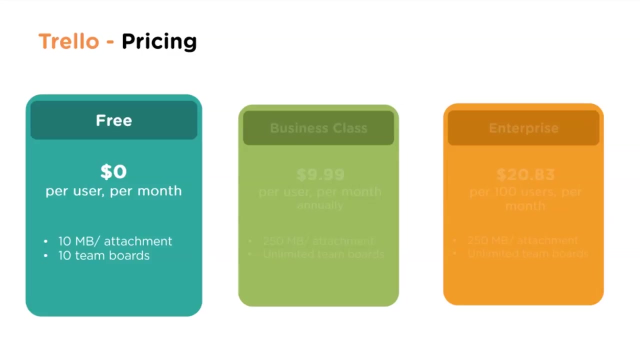 used by over 50 million people. the features of Trello includes smooth editing, easy file uploads from Dropbox or Google Drive, high security standards and easy data searching techniques. so the pricing includes: it is free for 10 MV per attachment and 10 team boards. business class includes 250 MB attachment, unlimited team boards and it. 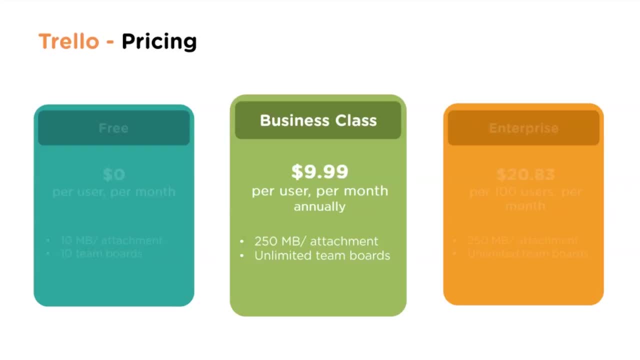 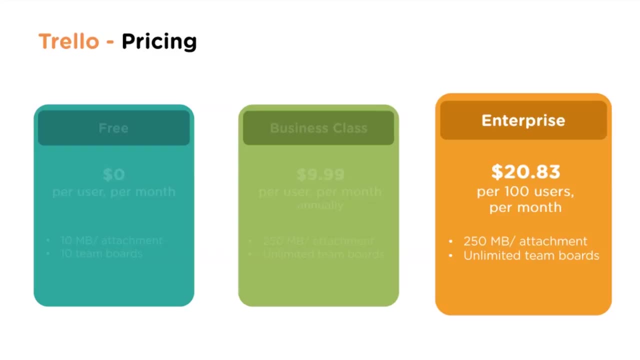 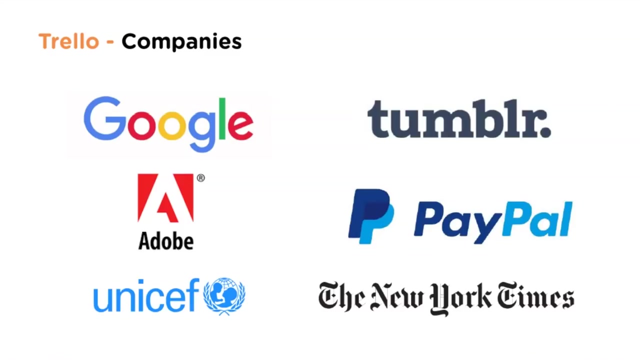 cost $9.99 per user per month annually. enterprise version provides 250 MB for attachment, unlimited team boards and costs around 20.83 dollars per hundred users per month. the companies who use Trello are Google, adobe, paypal, unicef, the New York Times, etc. now let us look at Asuna. the Asuna tool was released during the last 3 years. 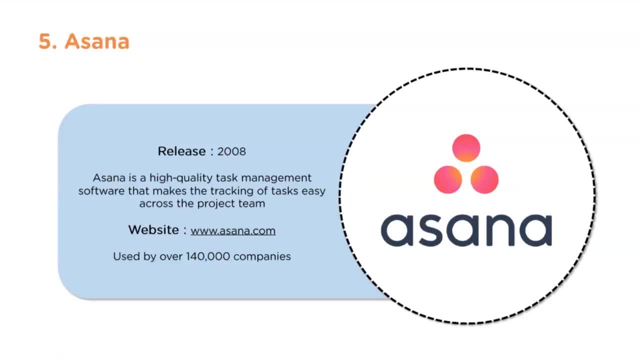 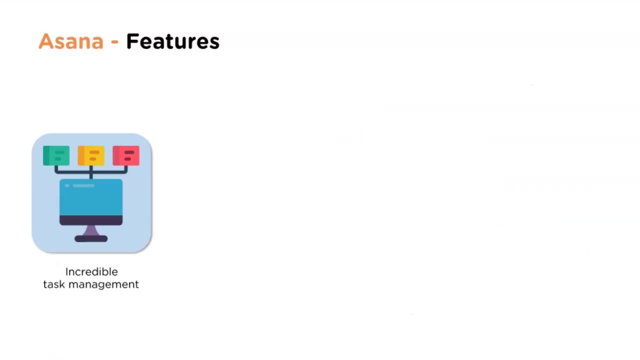 2008. it is an high quality task management software that makes the tracking of tasks easy across the project management. the website to access this tool is wwwasanacom, used by over 140,000 companies. the features includes incredible task management, Gantt charts, privacy controls easy. 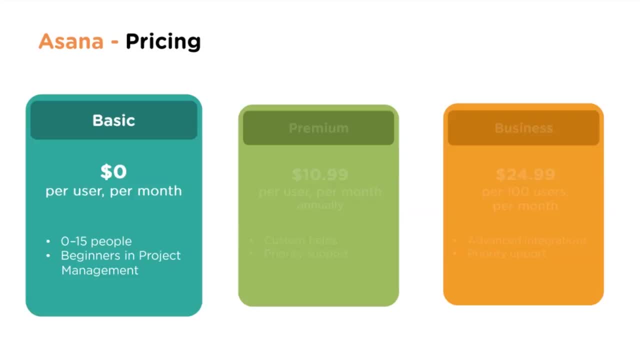 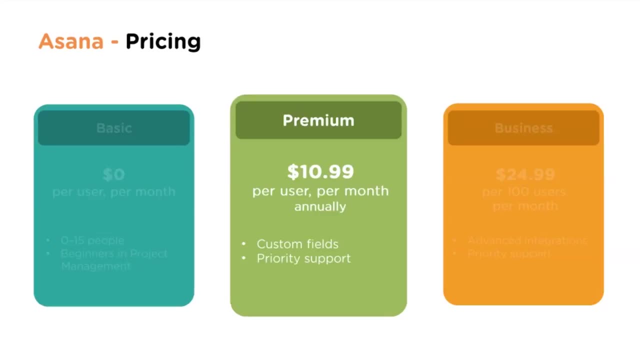 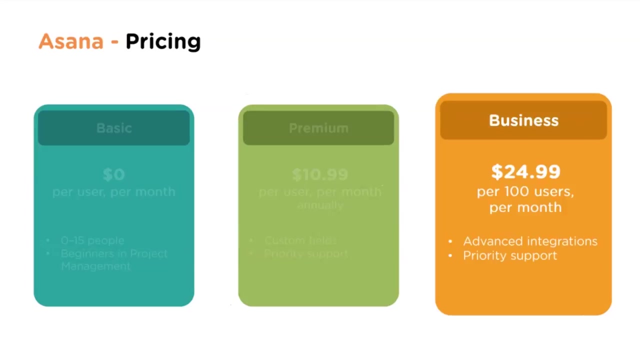 progress tracking. the pricing includes the basic model. asana is a provide 0 to 15 people beginners in the project management, so premium includes custom fields priority support where the pricing is dollar 10.99 per user per month annually. the business version includes advanced integration priority. 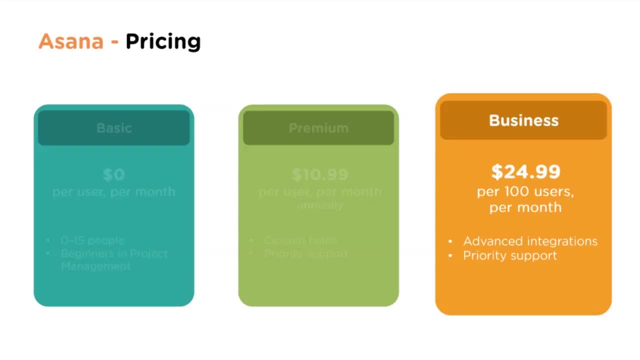 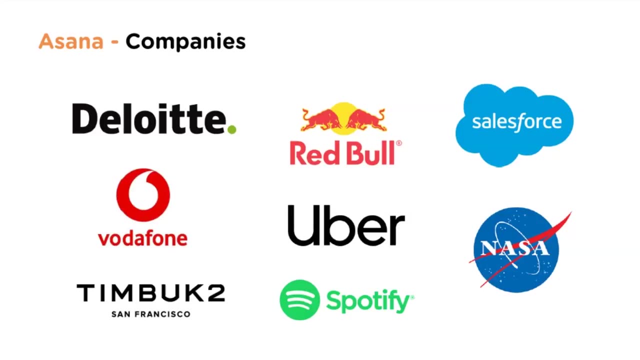 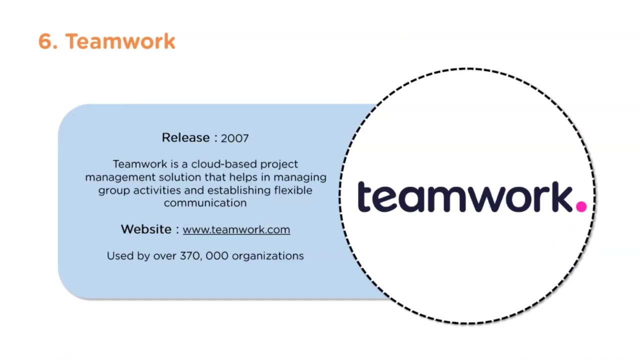 support and it costs twenty four point nine nine dollars per hundred users per month. the companies which uses asana are Deloitte, Vodafone, Red Bull, uber, Salesforce, NASA, etc. let us look at teamwork tool. teamwork was released during 2007. it is a cloud-based project management solution that helps in. 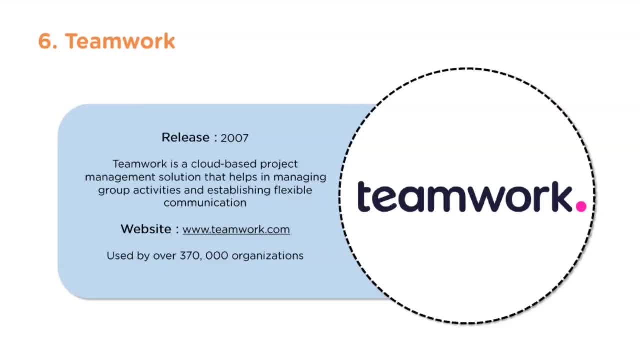 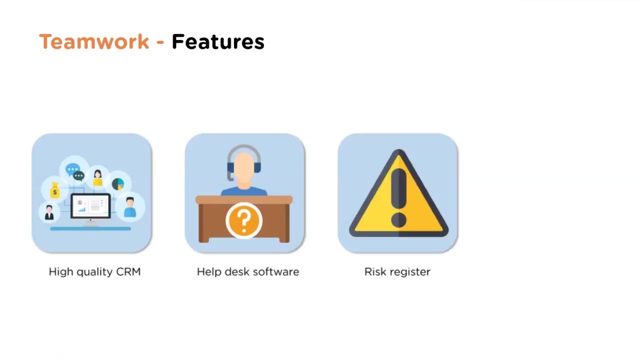 managing group activities and establishing flexible communication. the website to access this tool is wwwteamworkcom, used by over 370,000 organizations. the features of teamwork includes high quality CRM, helpdesk software, risk register and easy time tracking. the pricing includes 0 to 5. 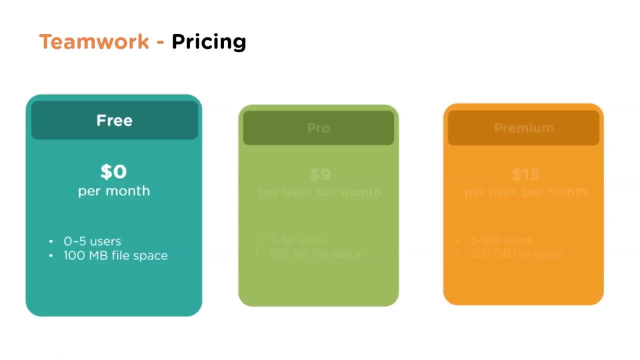 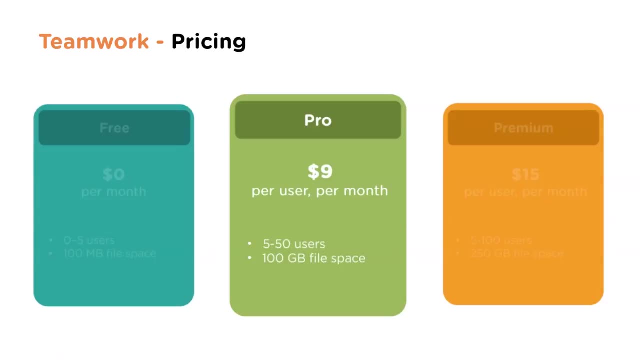 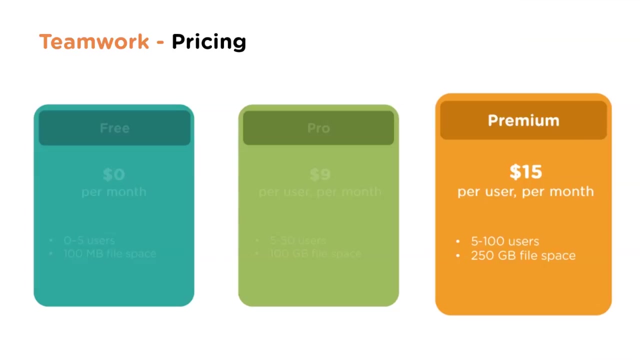 users and 100 MB file space is provided free of cost, whereas pro version includes 5 to 50 users under GB file spaces, which cost nine dollars per user per month. premium origin costs around dollar 15 per user per month, which includes 5 to 100 users and 250 GB file space. the organizations: 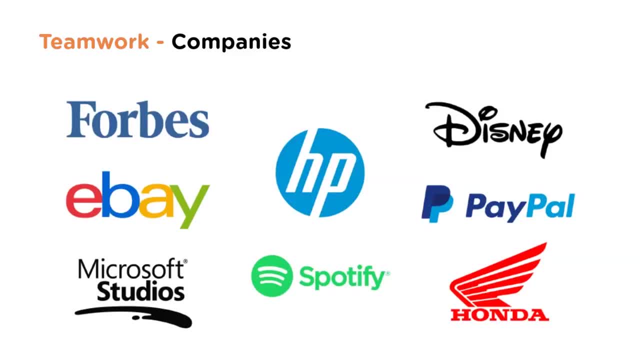 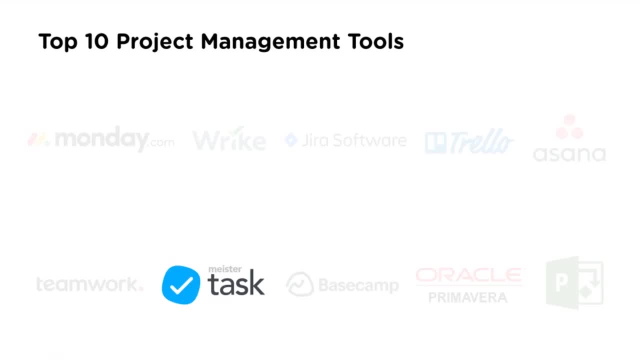 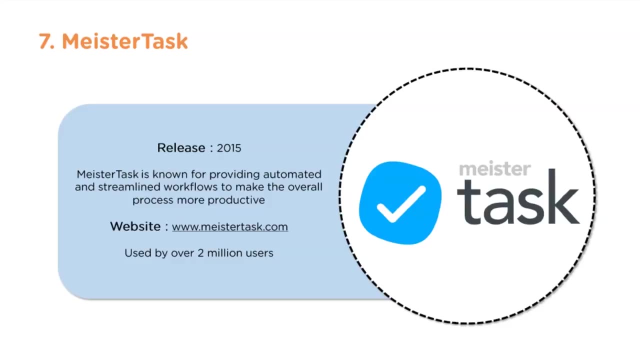 who use teamwork: czar, Forbes, eBay, Microsoft Studios, HP, PayPal, Disney's Honda. now let us look at the tool Meister task. so this tool was released during year 2015 and it is known for providing automated and streamlined workflows to make the overall processes more productive. the website to access. 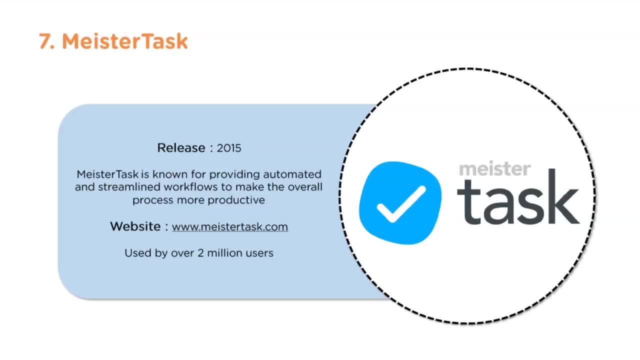 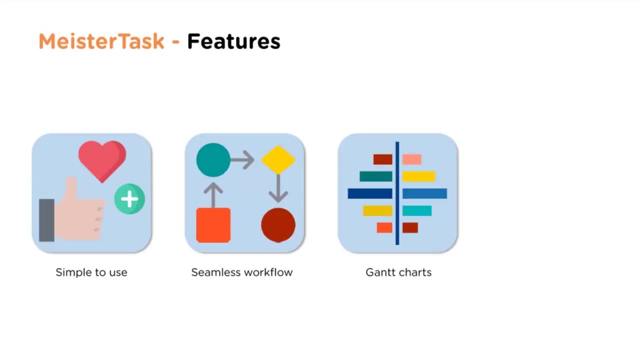 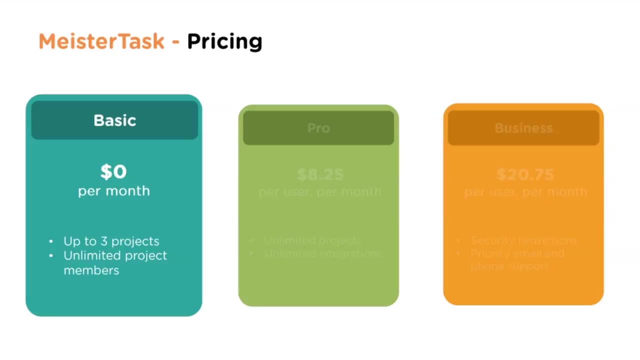 this is wwwmeistertaskcom, used by over two million users. the features of this tool includes: it is simple to use, seamless workflow, Gantt charts, flexible project boards. the pricing: it is zero dollars per month, up to three projects and unlimited project members. the pro version includes: 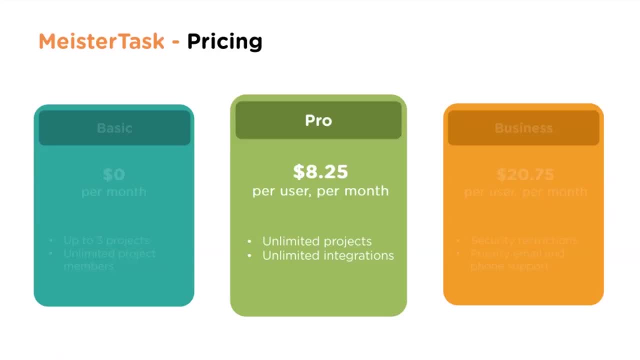 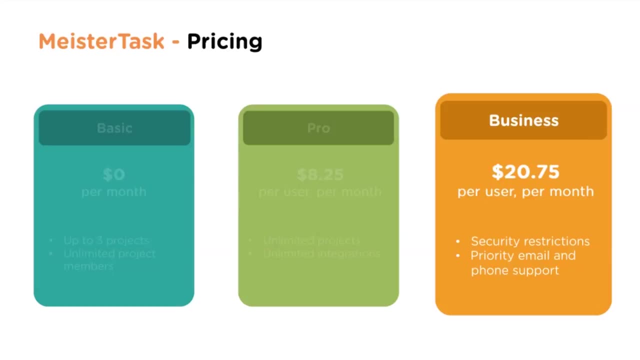 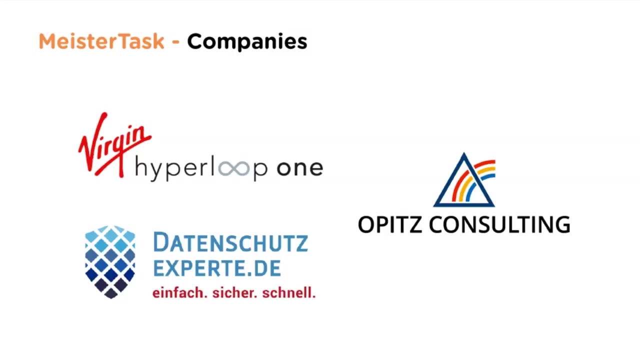 unlimited projects, unlimited integrations, which costs around 8.25 dollars per user per month, whereas business costs 20.75 dollars per user per month, which has security restrictions, priority email and phone support. the organization who use the tool are virgin optics consulting and datan. 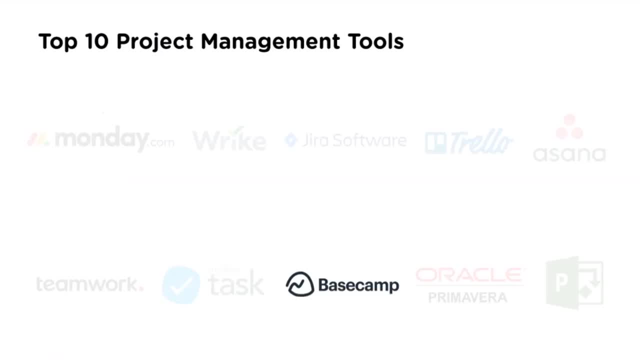 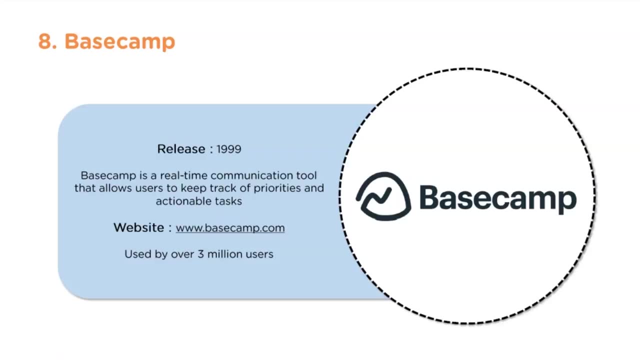 sukots, expert dot d, etc. basecamp: the basecamp tool was released during the year 1999. it is a real-time communication tool that allow users to keep track of priorities and actionable tasks. the website to access this tool is wwwbasecampcom, used by over 3 million users. the features of 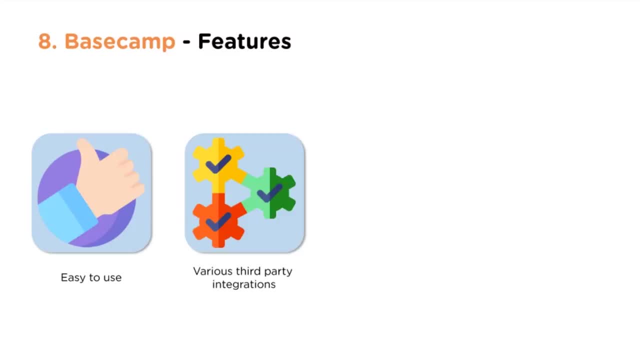 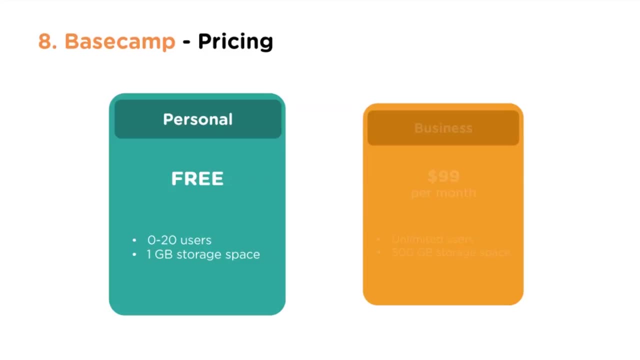 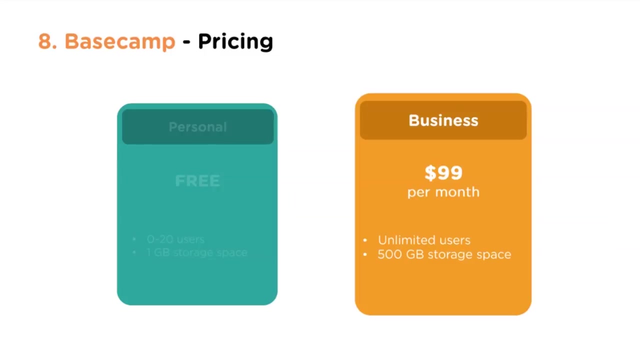 basecamp includes easy to use various third-party integrations, daily backups and comprehensive project calendar. the personal version is free and 0 to 20 users and 1 gb store space is provided. in business version it is 99.99 dollar per month for unlimited users having 500 gb storage space. the companies who use basecamp is 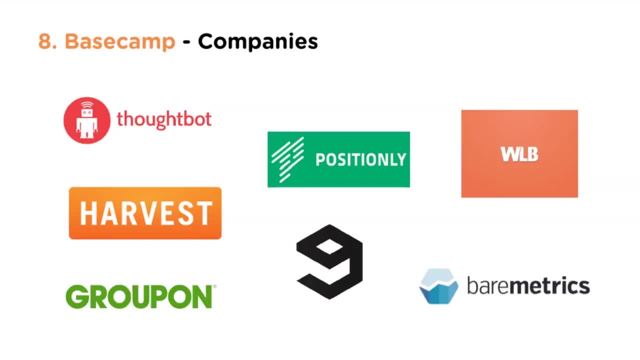 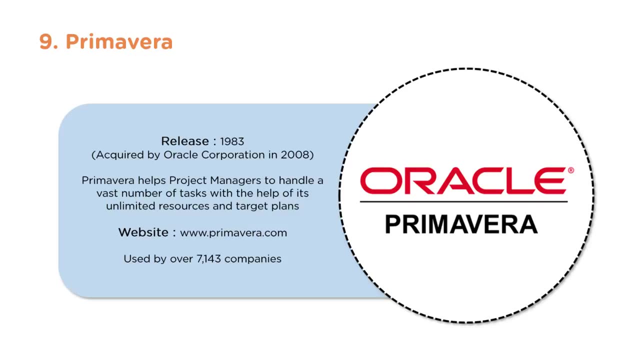 thoughtpot, harvest, wlb groupon, etc. oracle primavera. so this tool was released during the year 1983, which is acquired by oracle corporation in the year 2008.. primavera helps project manager to handle a vast number of tasks with the help of its unlimited resources and target plans. 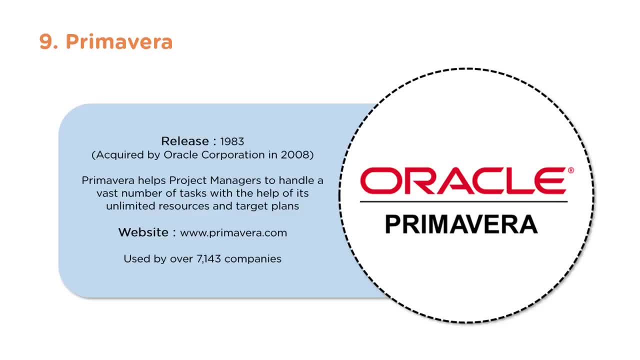 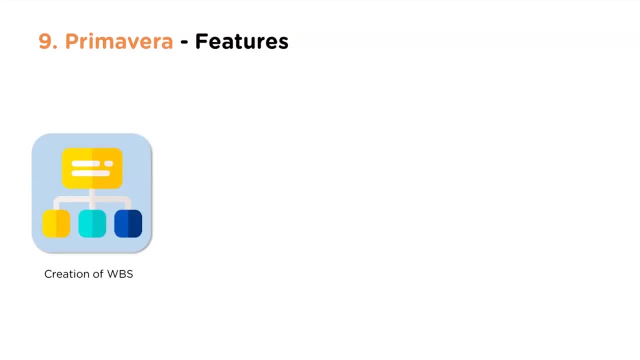 website to access this tool is wwwprimaveracom, which is used by over 7143 companies. so features of primavera includes creation of wbs. the work breakdown, structure issues and risk recording. supports large number of activities and easy collaboration with project users. the enterprise project portfolio management. 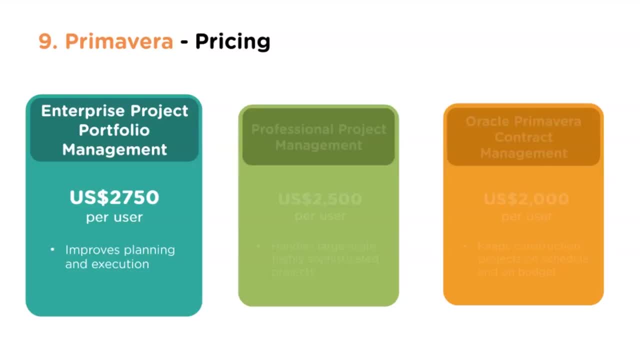 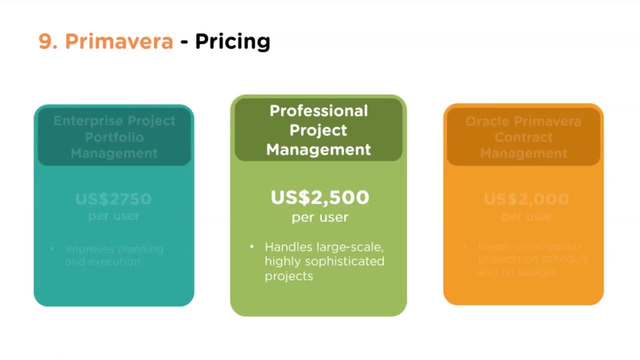 version costs around 2750 dollars per user, which improves planning and execution. professional project management version is USD 2500 per year and six month. chickens that are installed in your project is used to build dollar analytics. that works for project designs. user handles large-scale, highly sophisticated projects, so Oracle 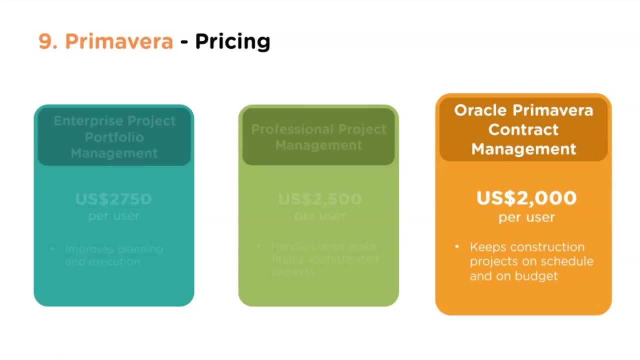 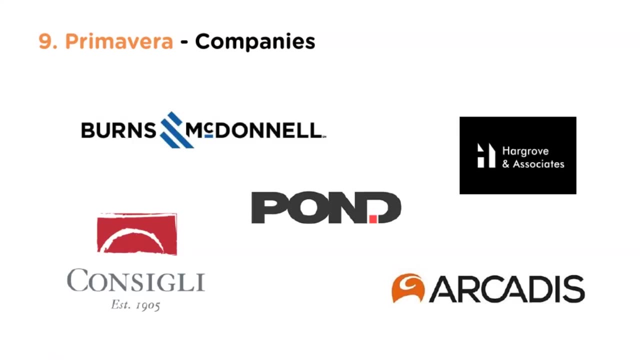 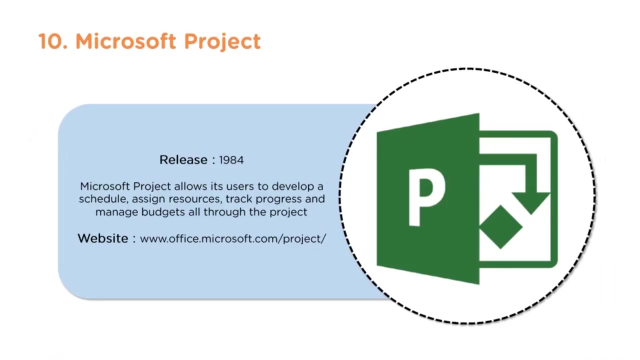 Primavera contract management version module costs around USD 2000 per user. keeps construction projects on schedule and on budget. so the companies which use Primavera are Burns, McDonald's, pond, Arcadies, etc. Microsoft project. so Microsoft project management tool was used during the year 1984. so this tool 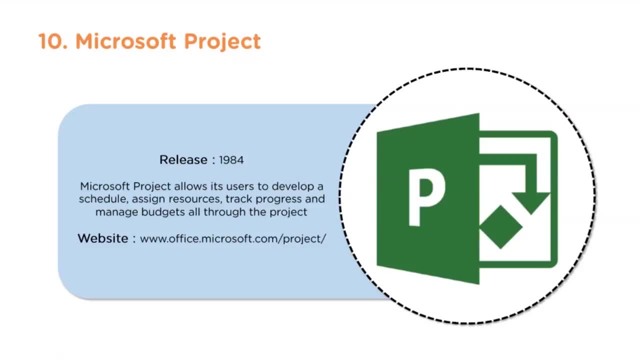 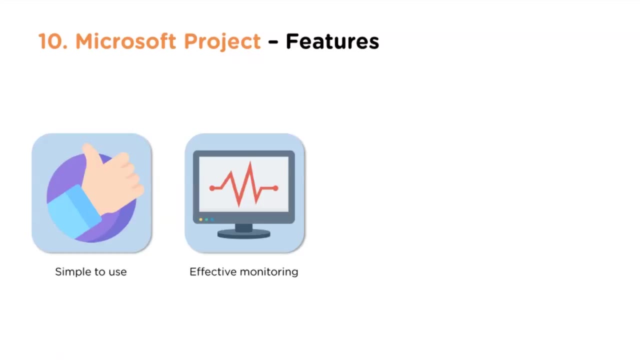 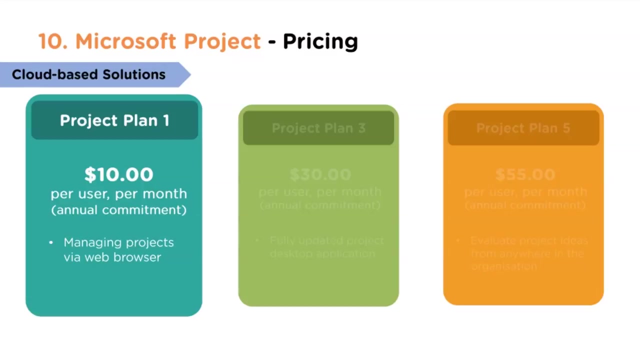 allows users to develop a schedule, assign resources, track progress and manage budgets all through the project. the website to access this tool is wwwofficemicrosoftcom slash project. the features of Microsoft project includes: simple to use, effective monitoring, easy communication, enhanced decision making. so this is a cloud-based solution and the pricing is project plan. 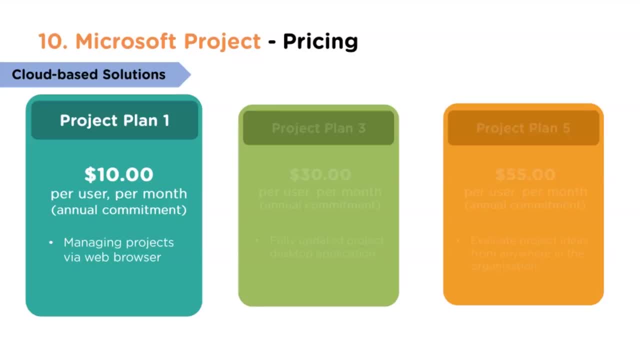 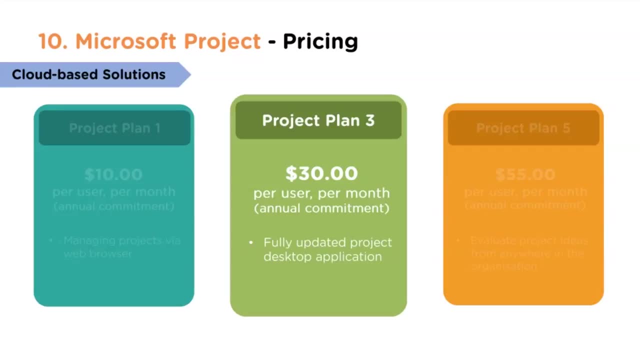 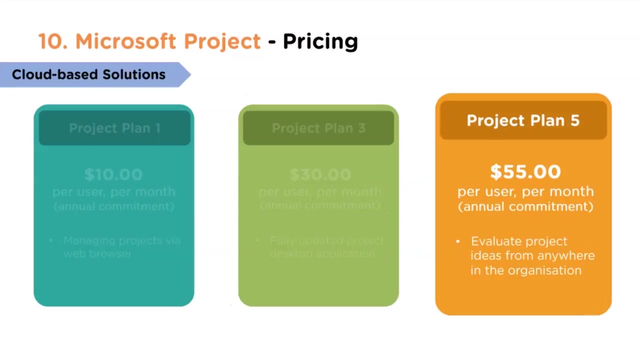 one costs around dollar ten per user per month on an annual basis commitment. Managing projects via web browser is the feature- Project plan 3- which costs around $1.30 per user per month with annual commitment, which is fully updated project desktop application- Project plan 5, which costs 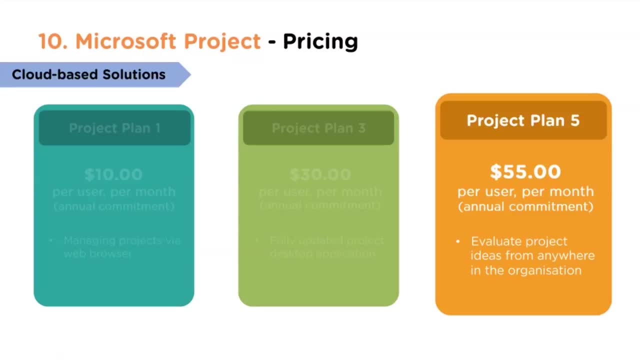 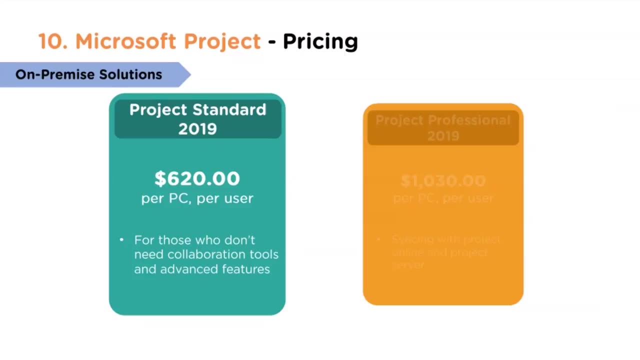 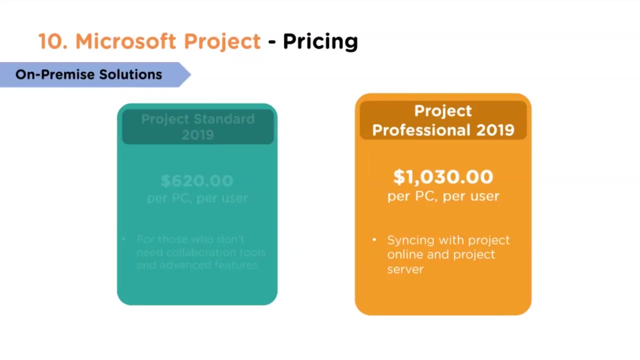 around $55 per user per month with annual commitment. Evaluating project ideas from anywhere in the organization is possible through this Project. standard 2019 version costs around $620 per PC per user for those who don't need collaboration tools and advanced features. Project professional version.